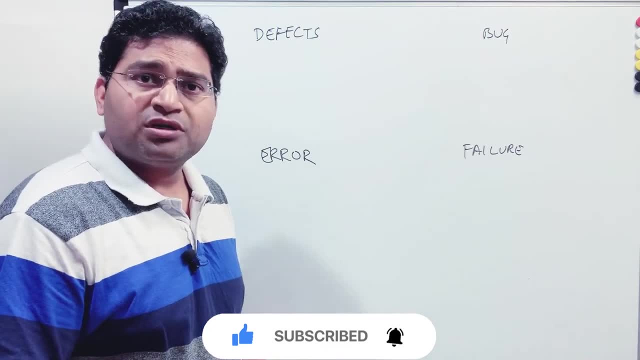 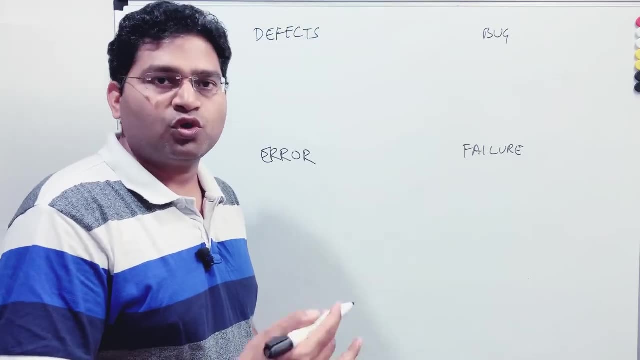 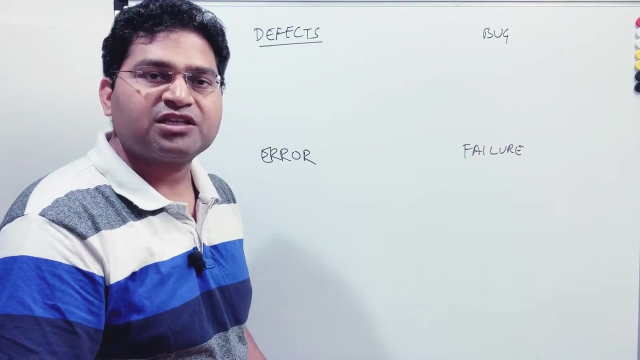 difference between these two. In terms of interview, it is important if somebody is, you know, looking for the difference, you can explain what the difference is, but actually in the real projects it won't matter much. So when we talk about defects, a defect is any deviation from the expected result, and same thing is. 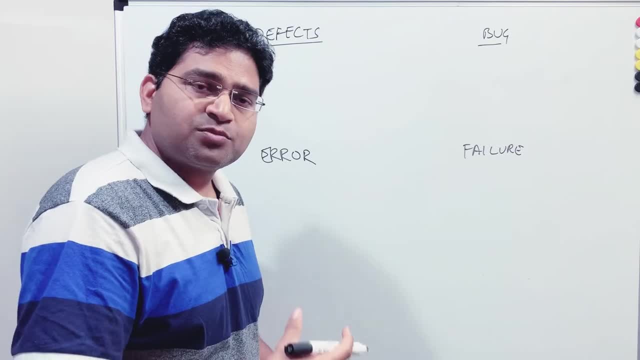 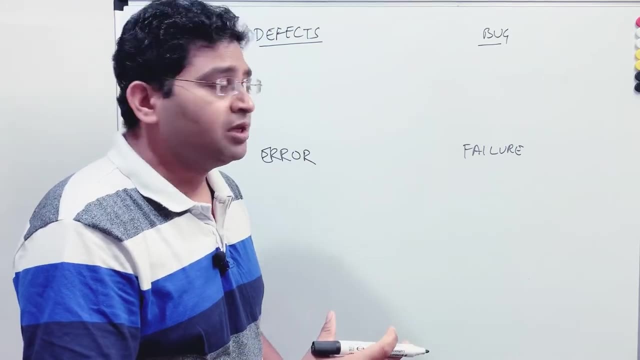 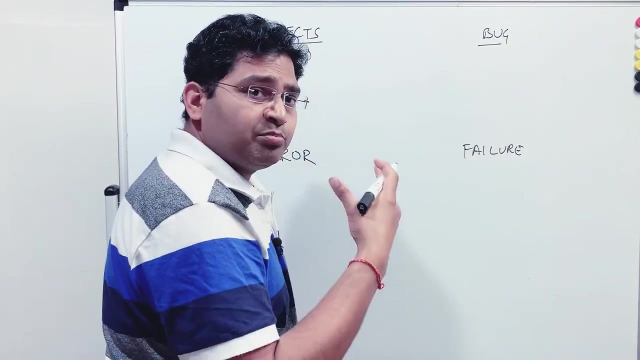 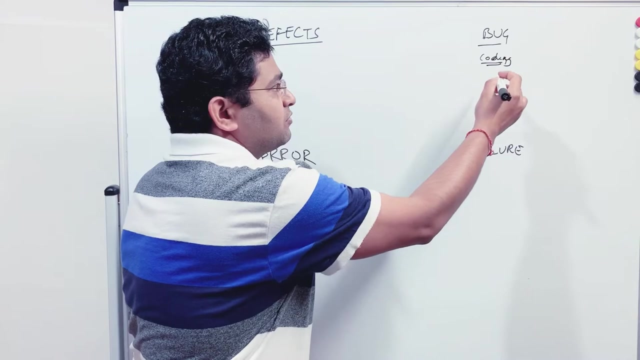 bug as well, right? So any deviation from the expected result is a defect or bug. So that is why they are used interchangeably. Now, a deviation is categorized as bug only if the failure is because of the coding error, So if the deviation is because of the 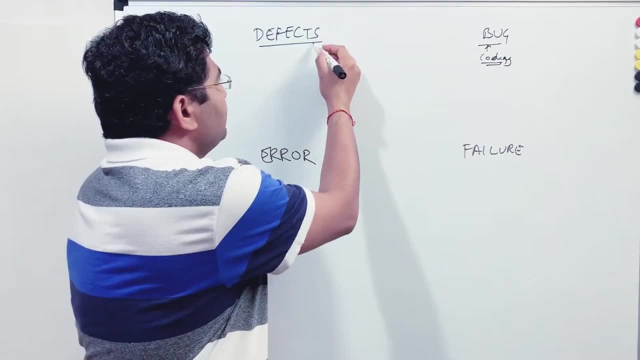 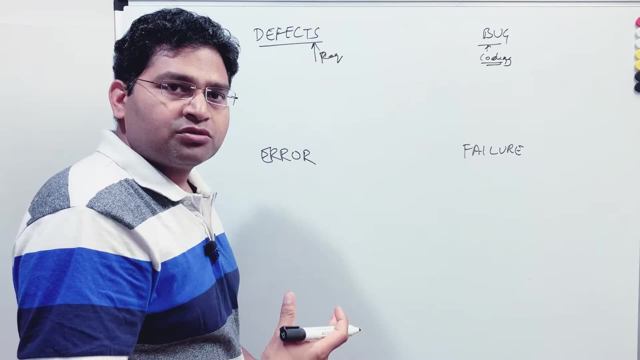 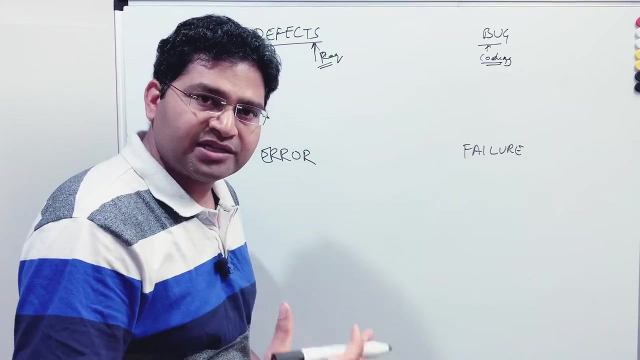 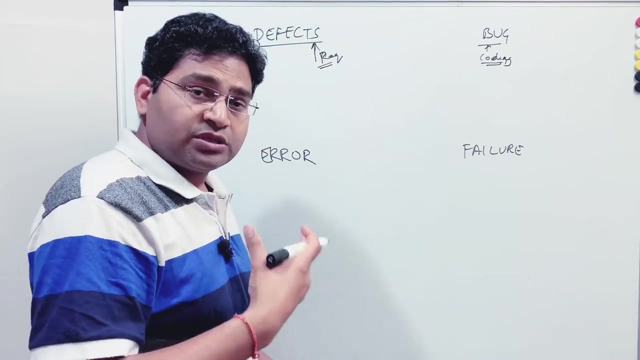 coding error, it is categorized as bug. If it is related to requirements- say, for example, there was missing requirement or misunderstood requirement and the actual outcome is not as per expectation because of the requirement issues or the requirement hasn't been met, then that is known as defect. so defects: for example, end user is going to is using the 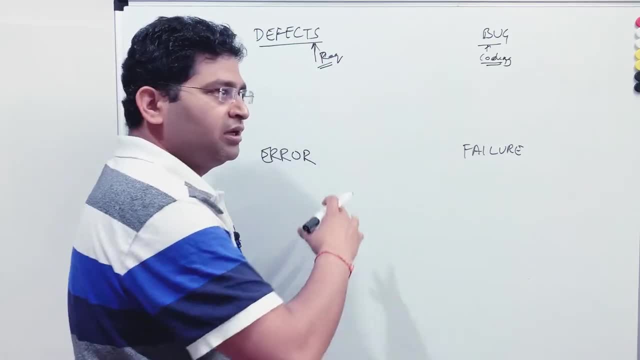 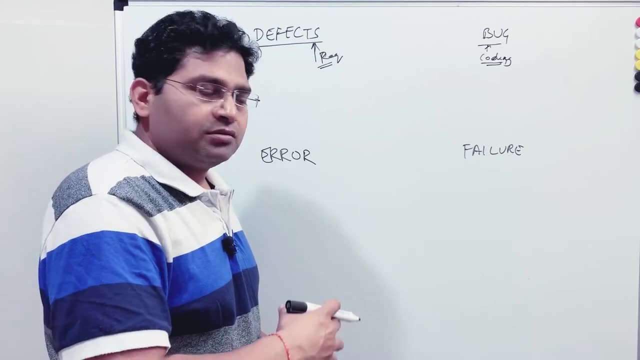 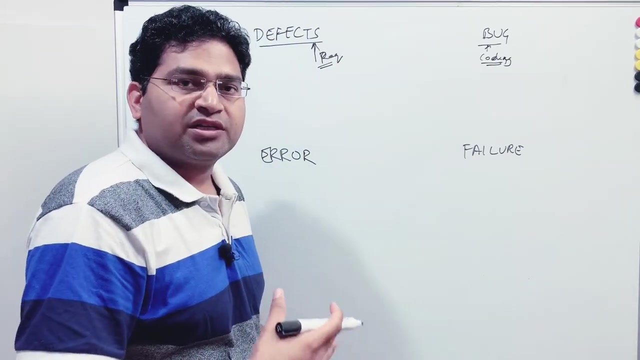 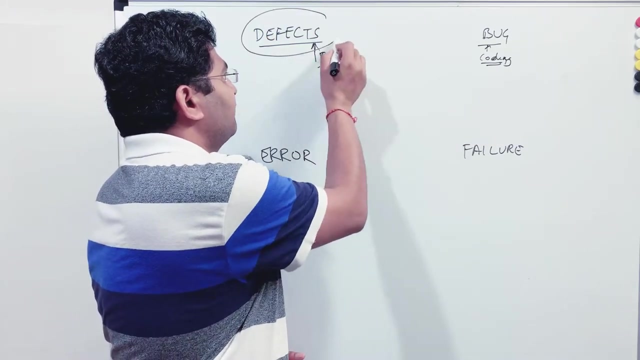 application and the requirement, whatever they have mentioned, that is not being fulfilled. even though the application is working- fine, it is, you know, there is no failure as such. still, the outcome is not as per expected requirement, then those sort of issues or the deviations from the expected results are categorized as defects. okay, however, if there is any deviation from the 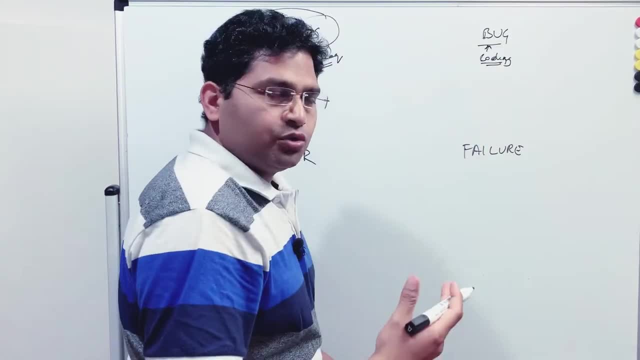 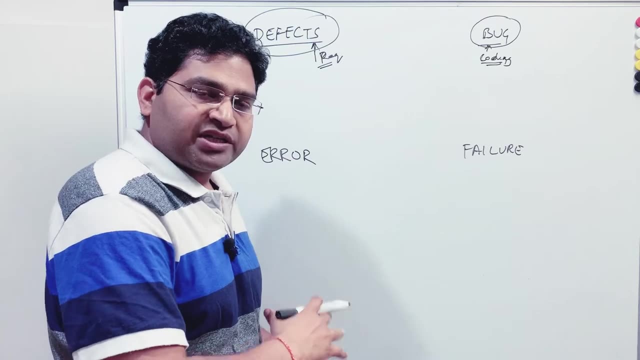 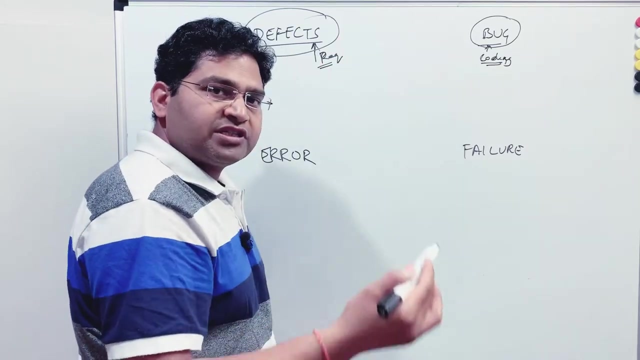 expected outcome because of the coding issues that is categorized as bug. okay, now, both of these are not as per expected requirement. then those sort of issues or the deviations from the These are the deviation from the expected result. So you can use them interchangeably In the actual tools. for example, you're using Jira. 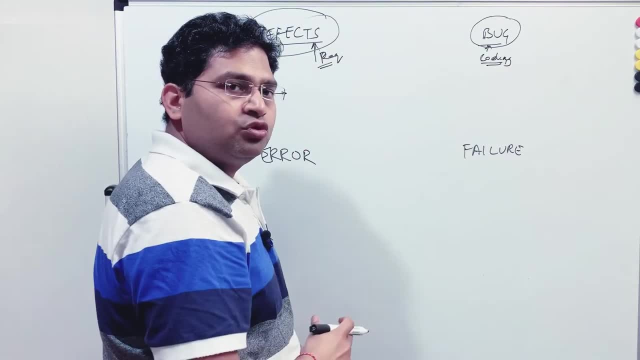 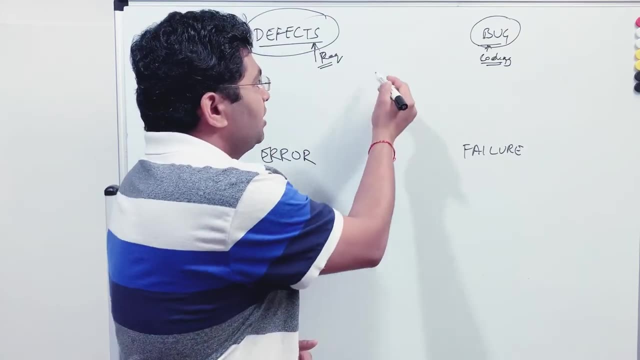 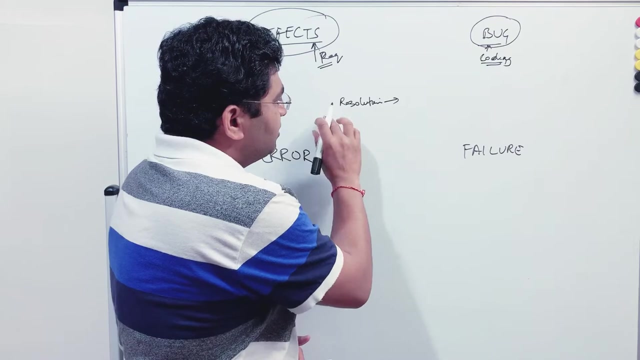 you will mostly be across the project or across the organization. you will be seeing these deviations either as defects or bugs or using them interchangeably. Within the tool there is a resolution field. So in Jira there is resolution field And once the issue has been raised, 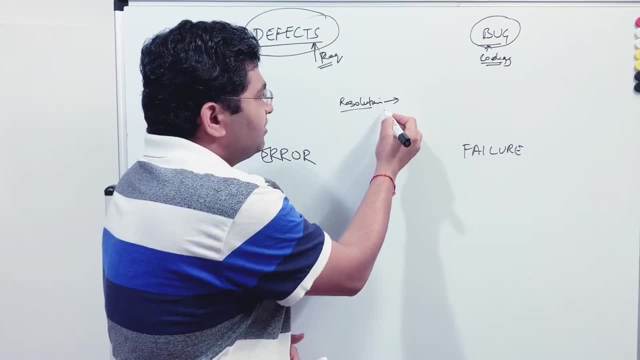 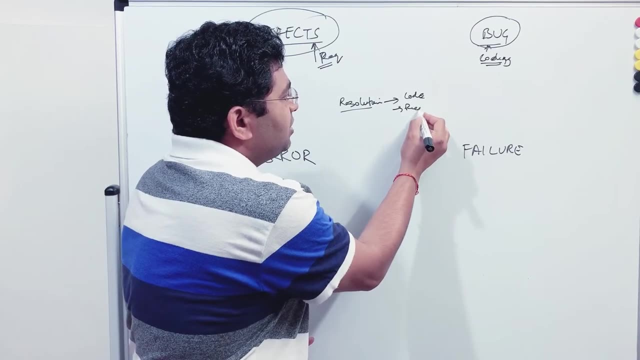 or defect or bug has been raised, when it is fixed or categorized, then in that case you mention whether the resolution is because of the code, or it is because of the requirement, or it is because of the environment, And this is what you will use: the resolution field. to categorize the defects or bug, Rather than having a separate category of defects and bug within the tool. you will be just using one term there, And that is why there is a lot of confusion between defects and bug. what is the difference? right? 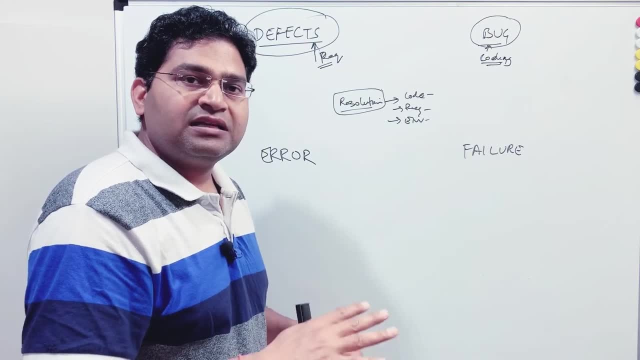 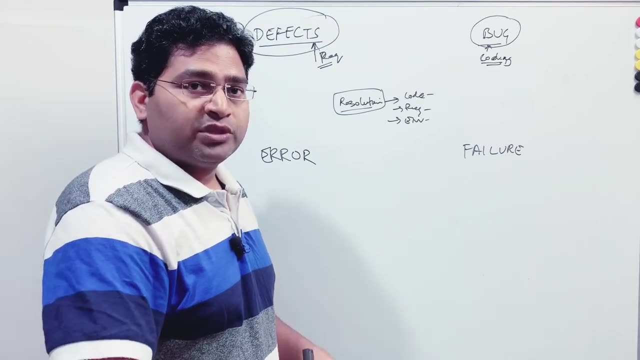 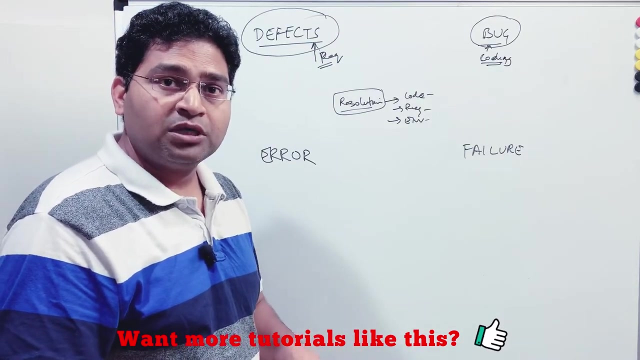 So there is such a minor difference that it is least bothered thing within the actual project. But in terms of interview, people are fussy about whether you know the difference or not. then you can explain this difference. It is least, it's going to matter least. 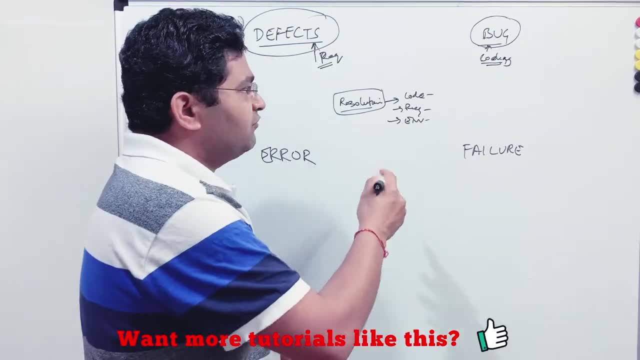 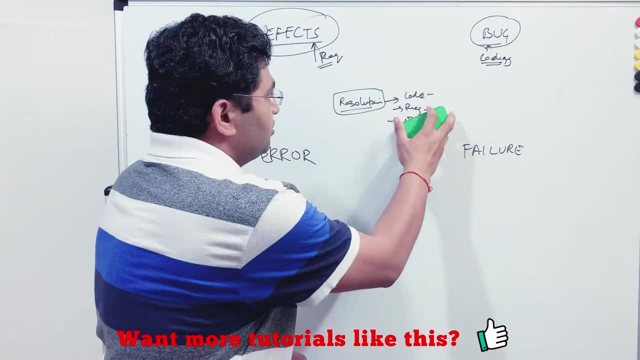 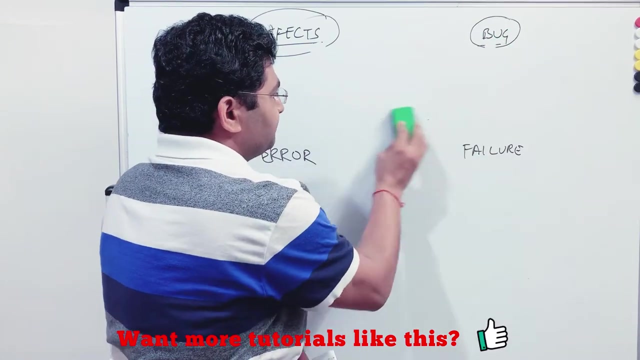 within the actual project when you are going to work. You have the resolution field and you have the categorization, so you can categorize these defects and bug. So this is the brief difference between the defect and bug And you can remember this in terms of interview purpose. 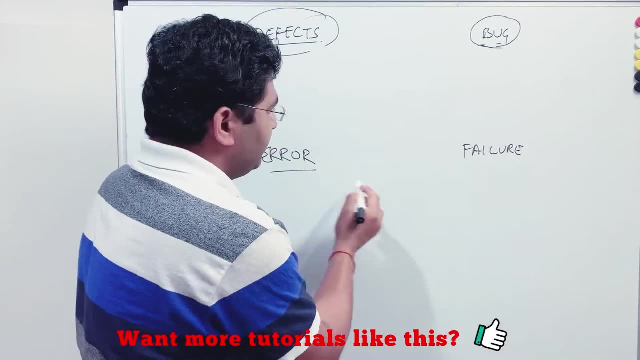 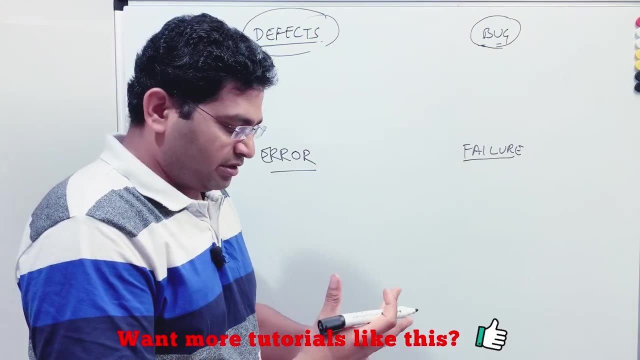 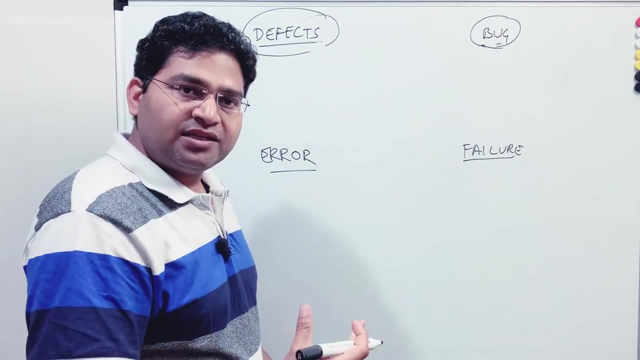 Now, when we talk about the error and failure, okay, So error is any error that can happen. So error in terms of capturing the requirement, error in terms of coding, error in terms of in terms of testing, When you are using the test data. 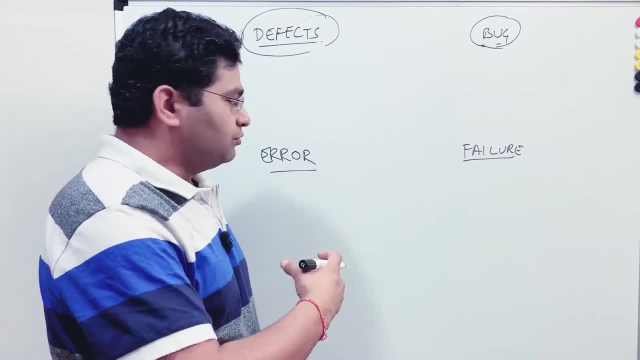 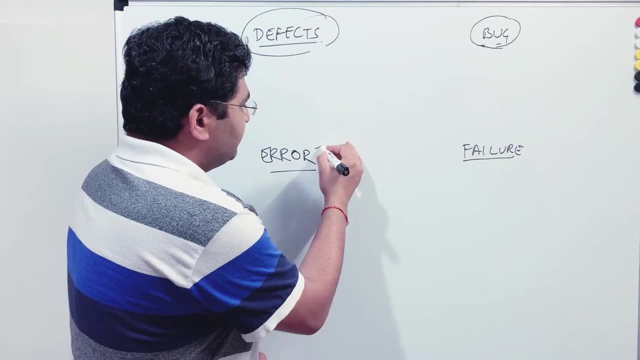 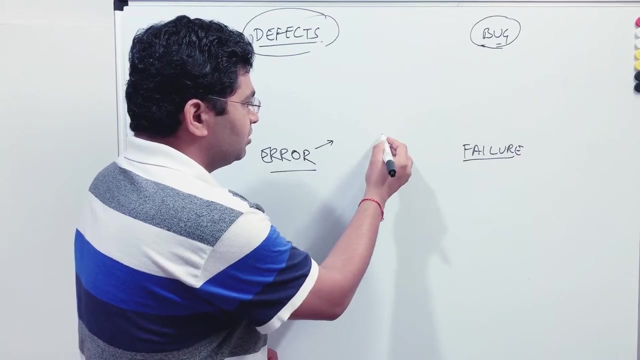 you might have used wrong test data, You might have tested using the wrong scenario, And any sort of error can happen. So error is it could be coding error. So, for example, within the code there is some error, So there was supposed to be, you know. 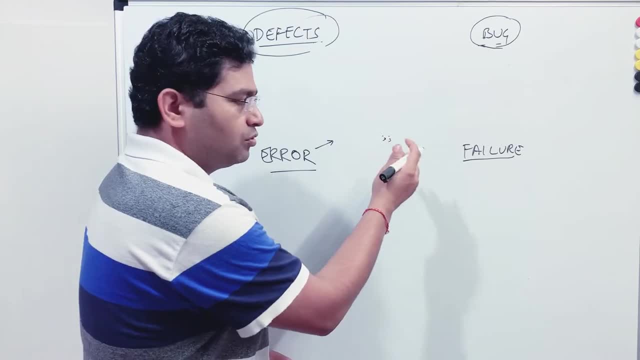 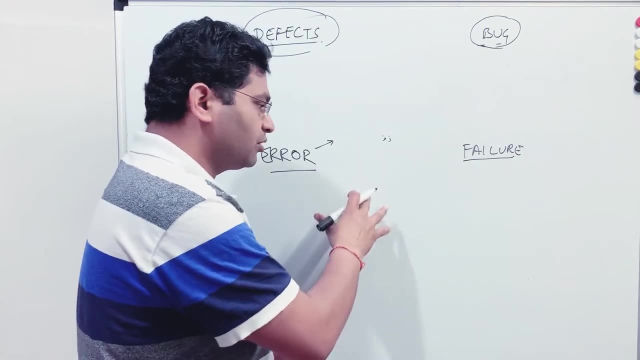 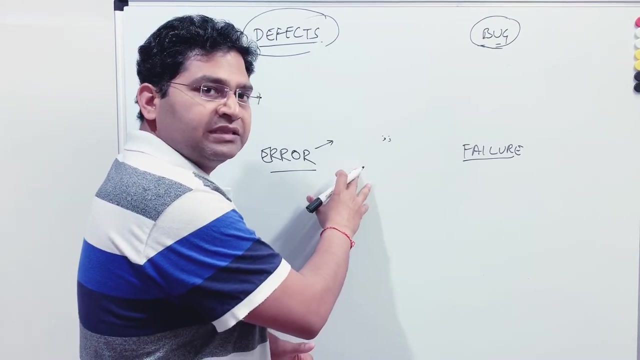 single colon. there have been two colon within the code Or there are. you know there is invalid return type. So any sort of error within the code or within the requirement capturing there can be error because of that invalid requirement that has been captured, the error requirement. 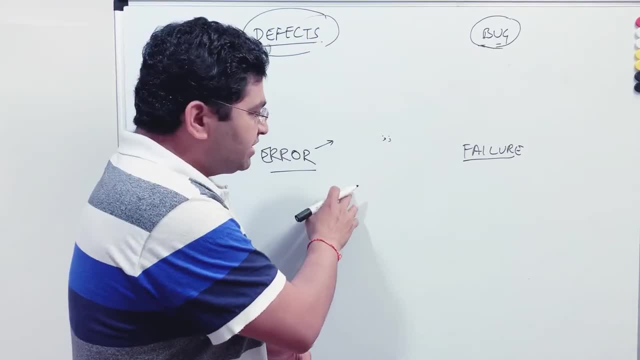 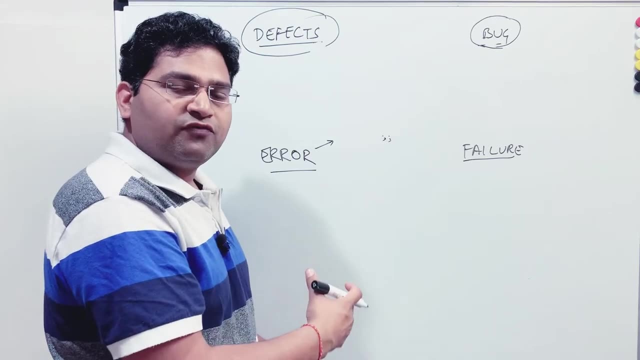 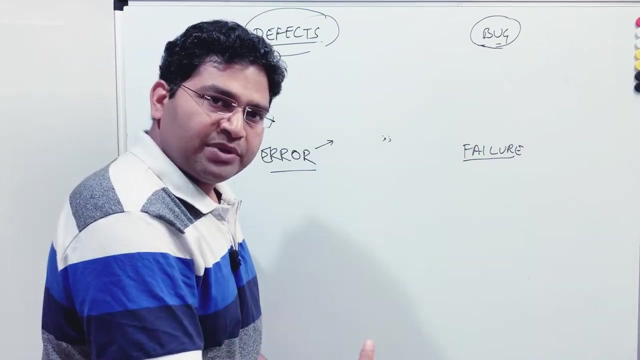 that has been captured, developer will implement that and which, in turn, will result in either defect or bug- right, so you know which- which in turn will anyways not fulfill what actual customer need are. so error is any error, whether it's requirement, whether it's, you know, development error or the test error. 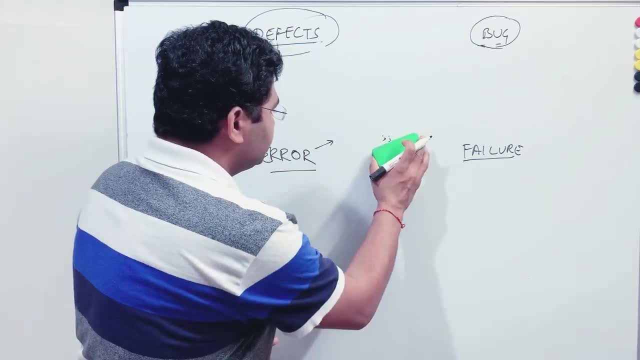 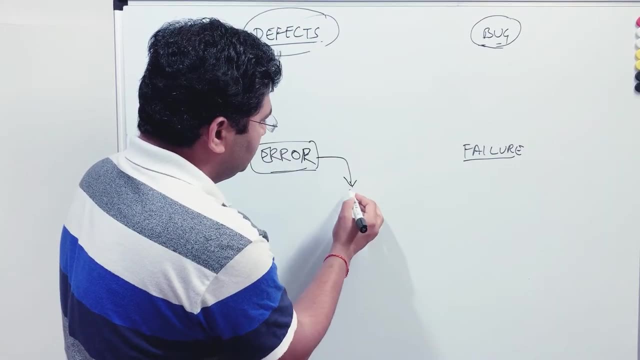 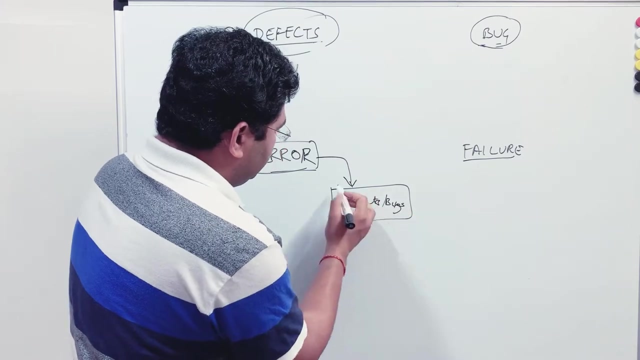 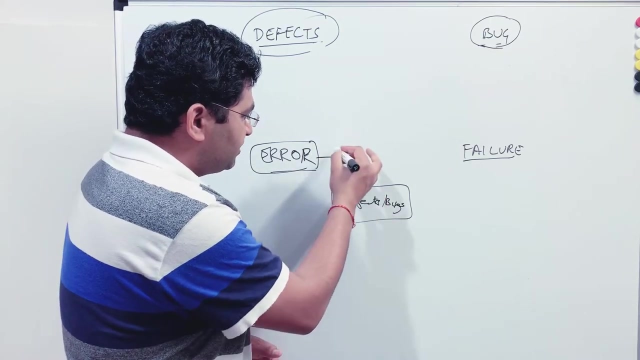 which leads to failure. okay, so how these terms are related. so usually error will lead to defects, right? so it will lead to defects or bugs as well, right? so whenever there will be error, whether it's in the requirement, whether it's in the coding, whether it's in the testing, so if it is in the test, in the coding, 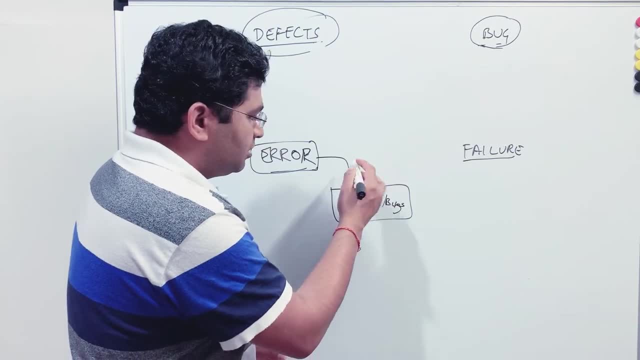 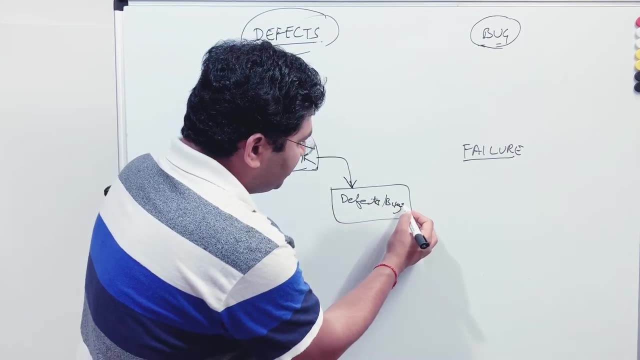 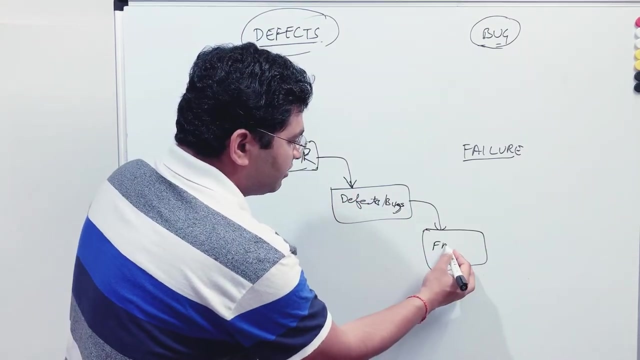 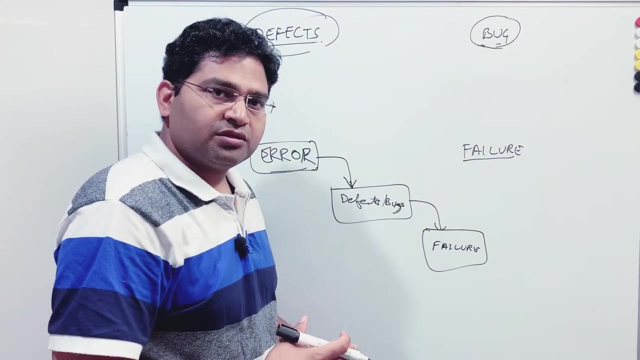 phase when you are going to test that particular deployed code, you will find the deviation from the expected result. so you will raise the defect and because of that defect or bug there is a failure, right? so if there is an error, only then there will be a failure. when we say failure, a failure is something which say: 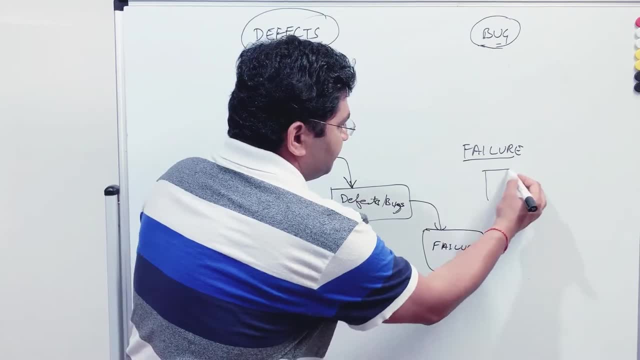 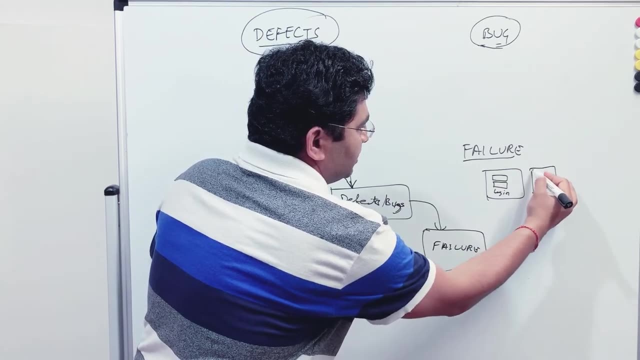 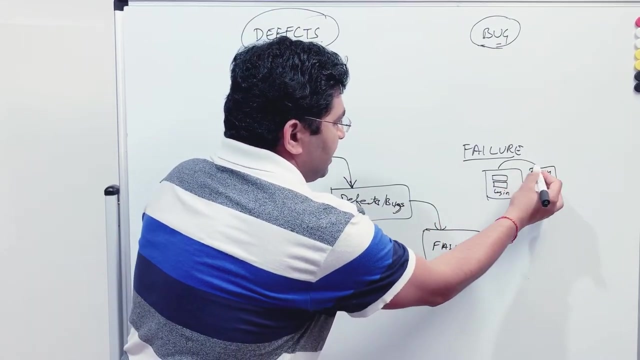 for example, in the login scenario, When I put username and password and click on login button, I should be able to redirect it or I should be on the dashboard page, right? so I should be on the dashboard page If this is not happening because of the error in the code. so when I put username and password, 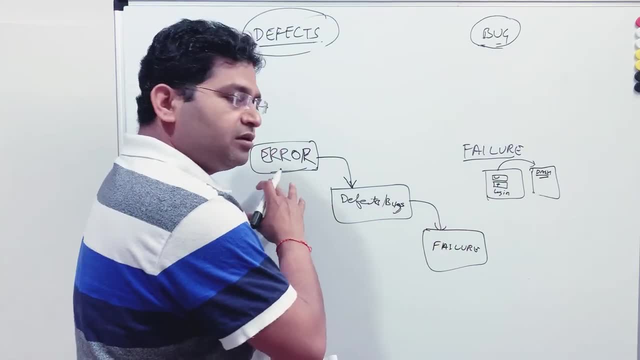 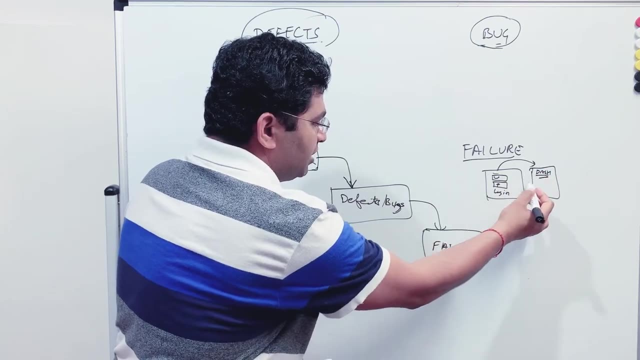 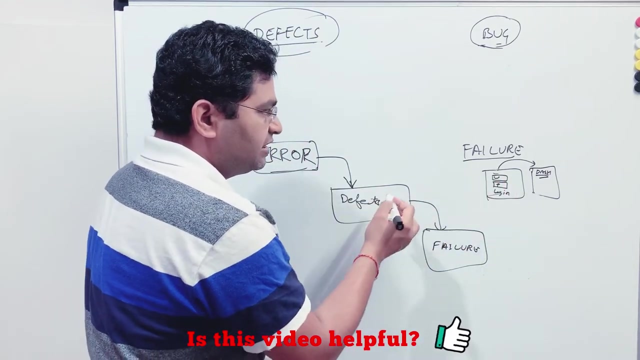 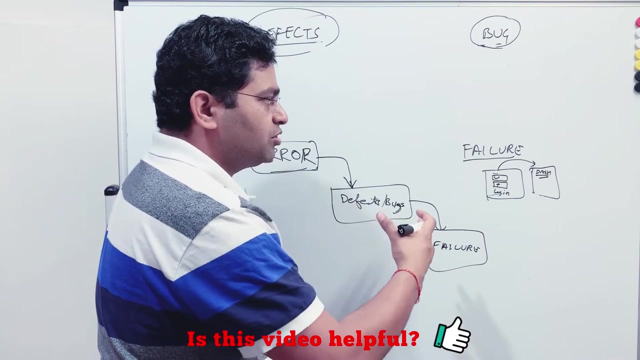 and click on login button. there was the error within the code. because of which error I couldn't be logged in successfully and the login is failing. So what this error resulted in? this code error resulted in the defect, and the defect is basically: I'm not able to. so the actual result is I'm not able to be redirected to. 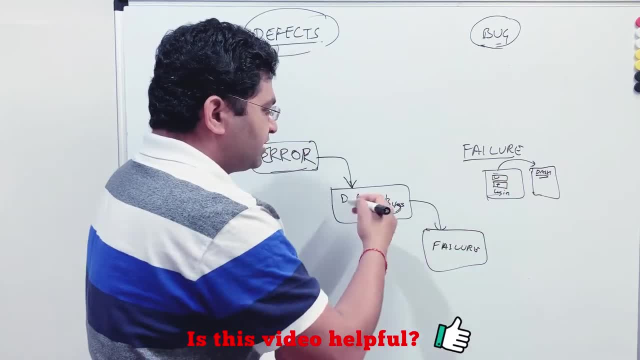 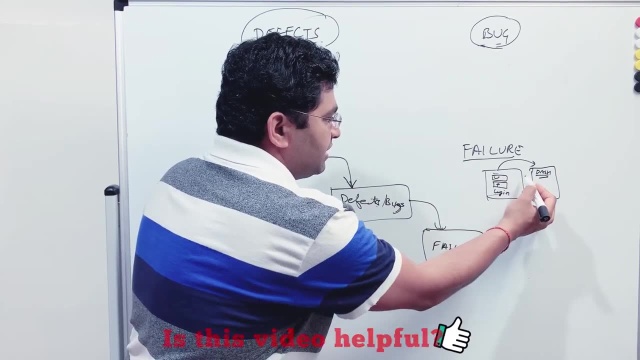 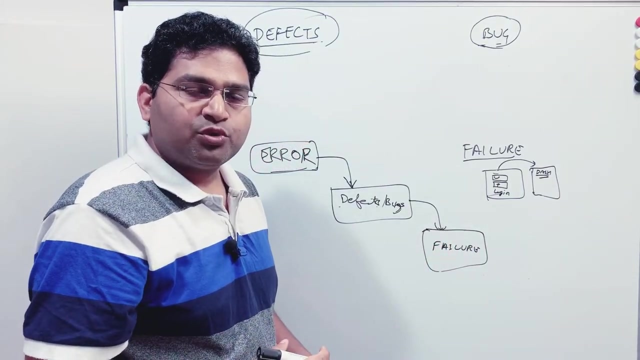 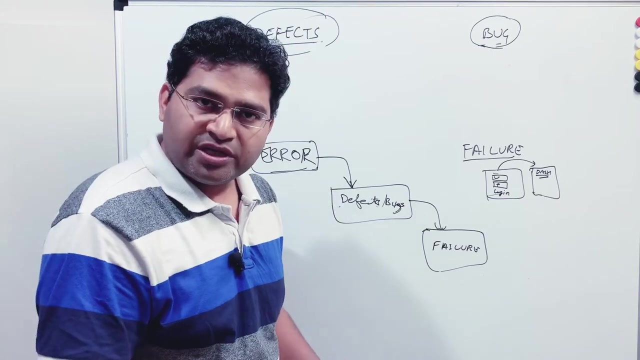 the dashboard page and which is not expected result. So which is the defect? and that defect caused the failure of me not logging into successfully and redirecting. So failure is the failure of what I'm supposed to actually achieve from the application. So it could be a blue screen failure. so in Windows, you see, many times Windows crashes. 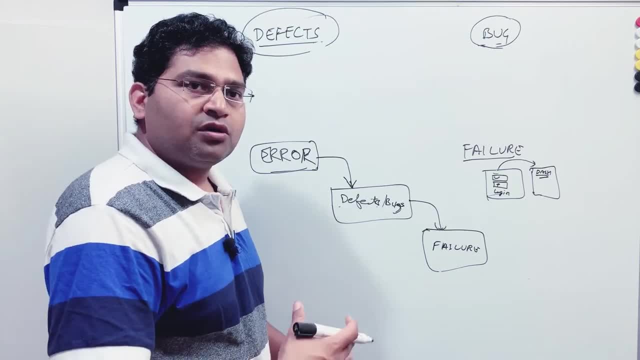 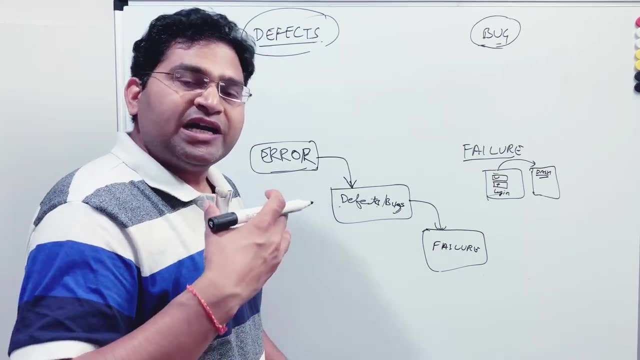 so that's a failure, and that failure is because of any error that is existing within the operating system code. Now, there might be error in the code, but that doesn't mean that it will not work. That doesn't mean that it will lead to failure all the time.